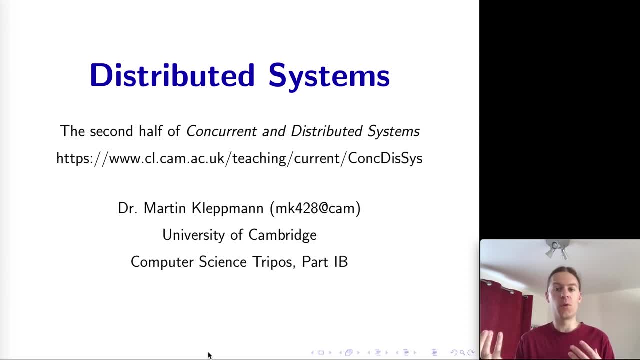 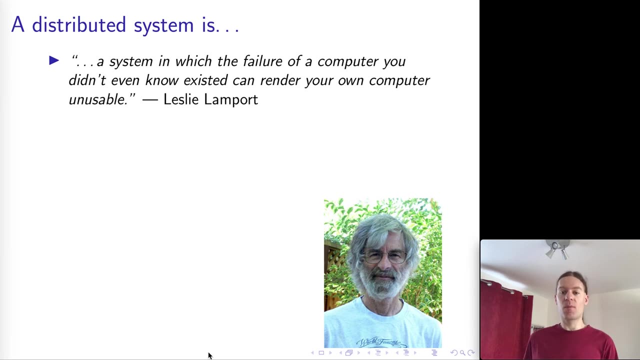 process. if you send it over the network to another process running on a different computer, that pointer will not necessarily make any sense to the recipient of that message, And so we have to think about different ways of sharing data between these concurrent entities. So a different. 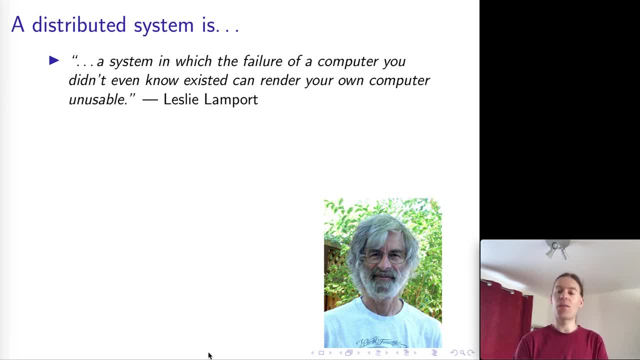 definition of a distributed system- somewhat joking definition- provided by Leslie Lamport, is that a distributed system is a system in which the failure of a computer you didn't even know existed can render your own computer unusable. Whether this is a good definition or not, we can debate. but 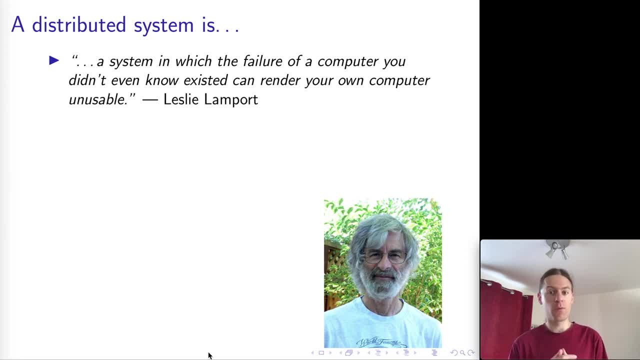 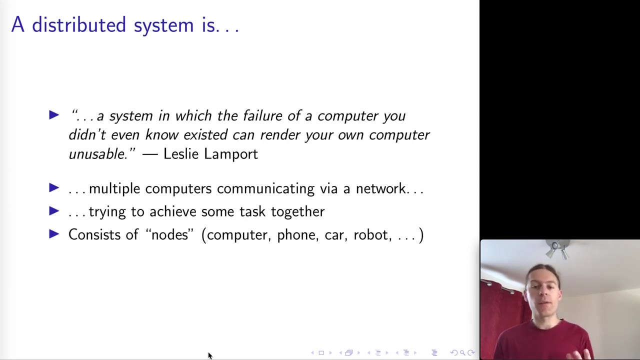 Leslie Lamport is a bit of a legend in the area of distributed systems and we will see various aspects of work that he's done over the decades. And of course lots of other people have done work in this area And we will see that over the course of these lectures. So, more generally, I think I would define a 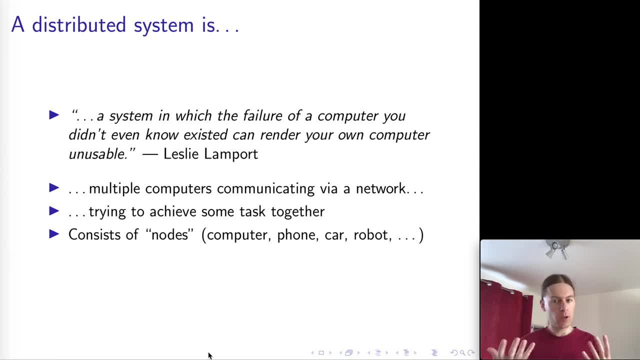 distributed system as one in which you have got multiple computers or computing devices. These devices might be smartphones, they might be robots, they might be self-driving cars, they might be desktop computers, they might be servers in a data center, So any sort of computing. 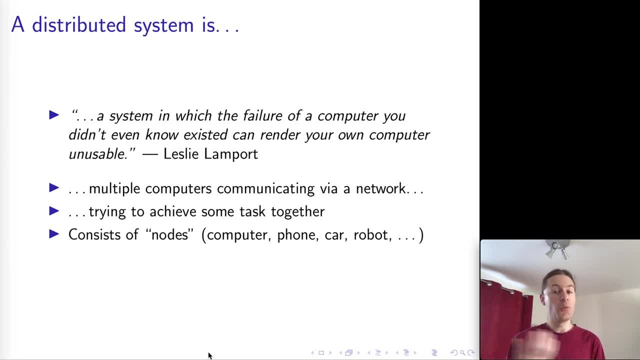 device really. And these computing devices are communicating via some kind of network, which might be a computer or a computer device, And these devices are communicating via some kind of network, which might be a computer or a computer device. And these devices are communicating via some kind of network. 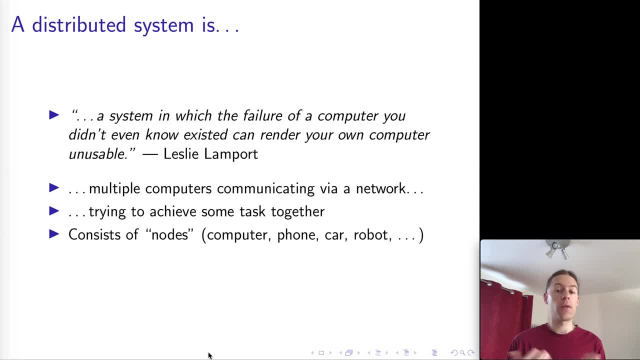 the internet and they are trying to achieve some kind of task together. And the study of distributed systems is really the study of how do we coordinate the activities of these different devices in such a way that they achieve together the tasks that they are trying to achieve. So I will start with. 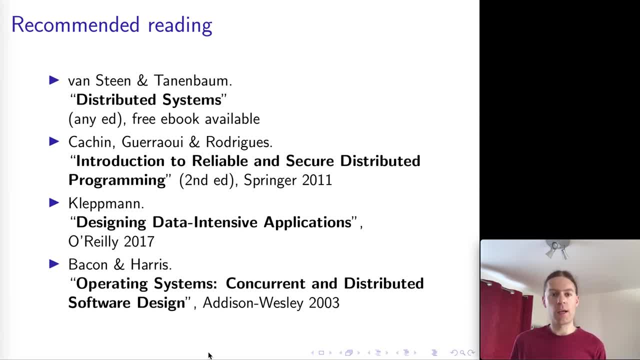 a little bit of background First, just the administrative things to get that done. So first of all, if you want any further background reading on this course, hopefully you'll be able to. the lecture notes will be reasonably self-contained, but of course further detail is available in books. 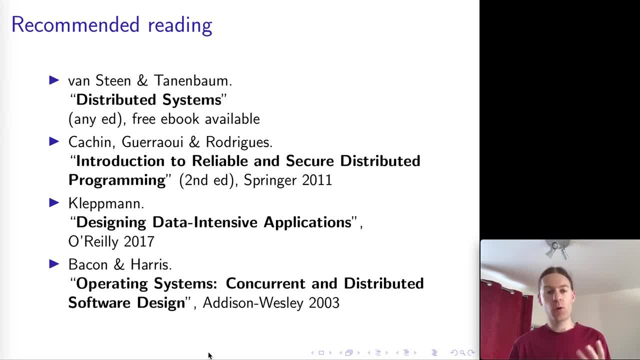 if you are interested, There are several different styles of books that I've put here on the list. So the textbook by Van Steen and Tannenbaum is a sort of systems level overview. So this is. it comes at distributed systems from quite an applied angle of real applications, that real 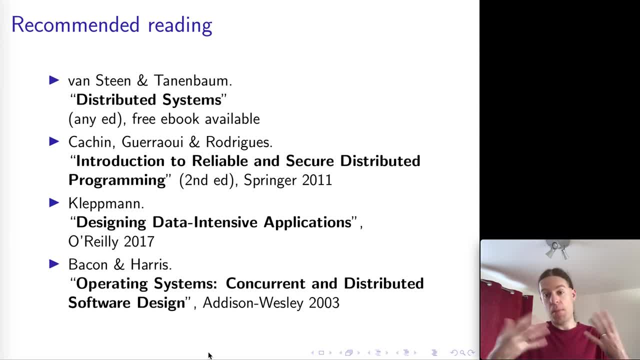 people use and discusses how these work and discusses how they work and how they work. This is the various implementation details of it. It doesn't go as far into the theory as some of the other books, but it's more practically oriented. If you like the theory, then the second book on 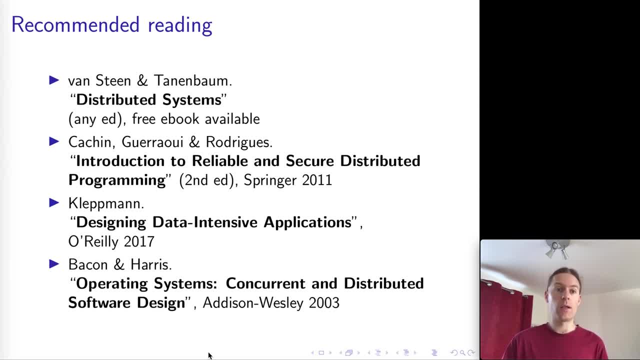 this list is a good choice. So the textbook by Kachin, Guerrari and Rodriguez is an excellent but quite detailed overview of distributed systems theory. So it goes into a lot more depth than we have time to talk about in this course. But if you want to read more about the theory, this is an 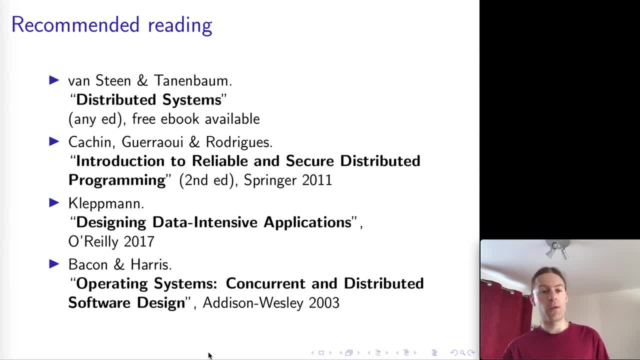 excellent book. There's another area called designing data intensive applications. This book is a bit more oriented towards distributed database systems, So it's not just not just distributed systems in general. There's a lot of other databases content in there, but it's- and this book is- more oriented. 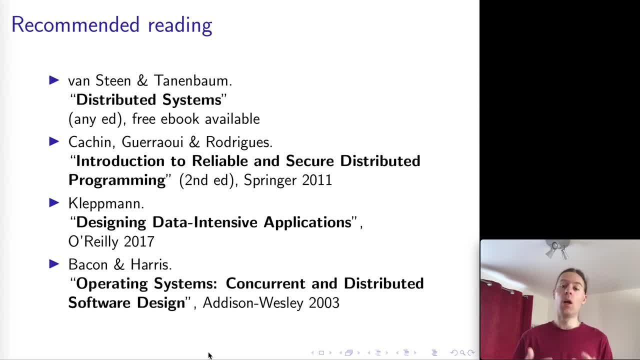 towards industrial software engineers. So people who are working professionally with distributed databases will probably find this kind of book useful. And finally there's the Bacon and Harris textbook Which was already recommended for the concurrent systems part of this course Which really provides the link between operating systems and distributed systems. 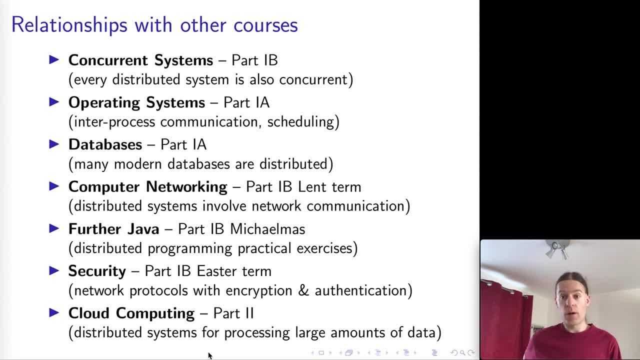 Okay, so this course is also connected to various other courses in the tripos, Most obviously concurrent systems that this course is part of, Also operating systems, which you studied last year. So all of the background that you have there on processes and inter-process communication. 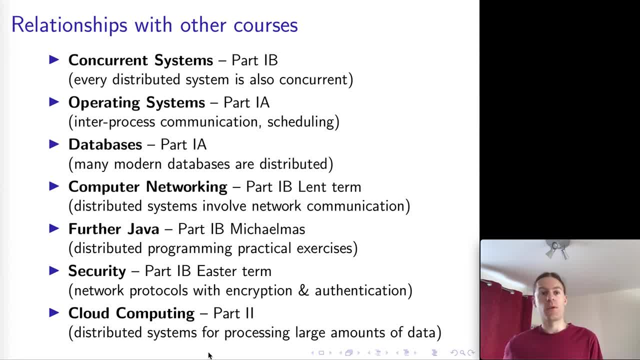 and scheduling of processes. all of that stuff is relevant for this course. Also, the databases course is connected to distributed systems Because, as I mentioned just now, many modern databases are in fact distributed and they use a lot of the techniques that we will talk about in this course. 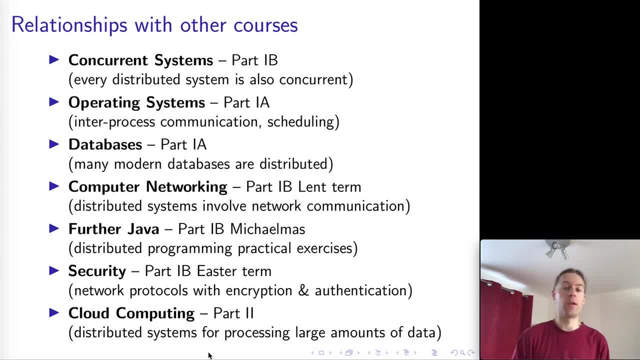 And so using modern databases often involves using distributed systems as well. there's a strong connection between distributed systems and computer networking Because, as I said, distributed systems involve network communication generally. The difference between the two courses is that the computer networking course is mostly about how do you actually get the bytes over the wire from. 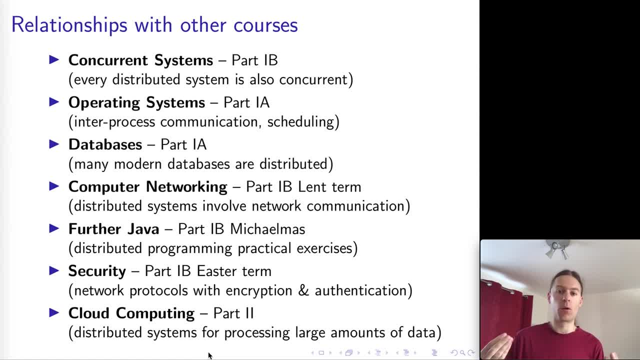 one device to the other device. So what do the network protocols look like that enable devices to communicate And then distributed systems builds on top of computer networking and saying, okay, assuming we now have this mechanism for devices to communicate, how can we now ensure? 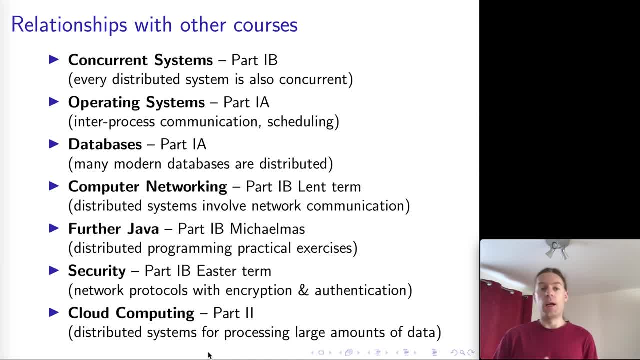 that these devices behave in the ways that we want. There's connection to further Java, So there's programming exercises that involve a bit of distributed computing. The security aspects of distributed systems are very interesting and they are covered in a course in Easter term, that's. 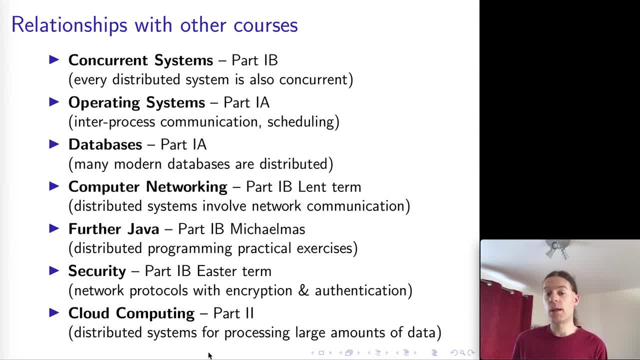 dedicated just to the topic of security. And finally, next year's cloud computing course builds upon distributed systems, because cloud computing is all about being able to flexibly process large amounts of data, And if you want to learn more about cloud computing, you can go to cloudcom. 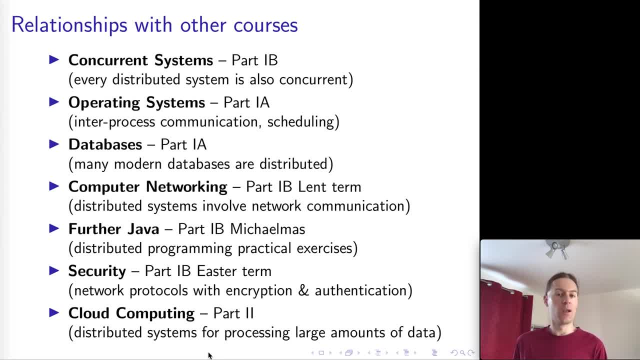 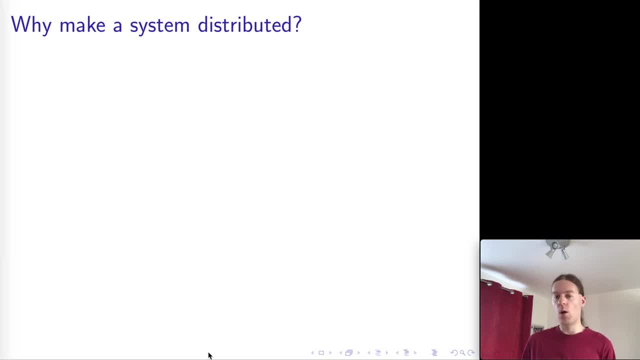 sufficiently large amounts of data, you generally need a distributed system in order to process it. Okay, so I gave a brief definition of what a distributed system is. The next question is then: why, Like why, should we go to all of this effort of making a system distributed? Why can't we just 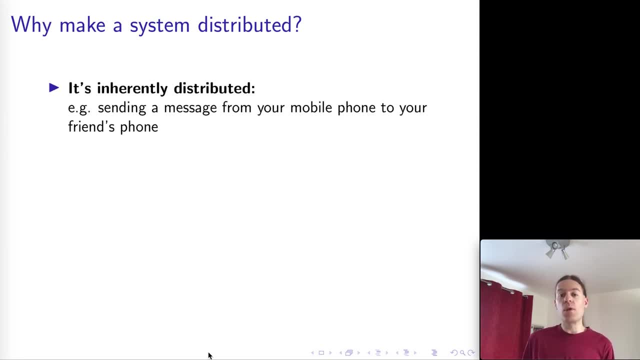 use a single computer and keep things simple. And well, one reason is that some applications, some types of things you want to do, computers are inherently distributed. So if you want to send a message from your phone to your friend's phone, this inevitably involves two different. 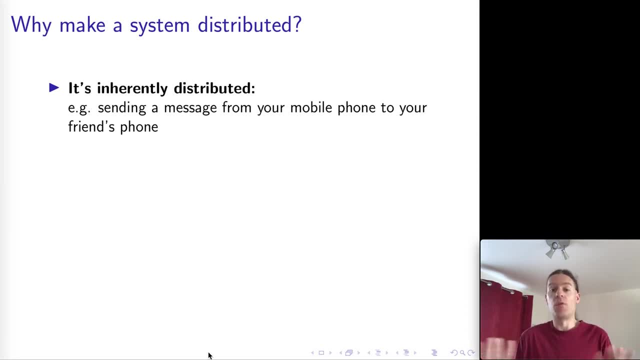 phones and a network, So this is a distributed system. There's no way around it. There's no way of building a messaging system that is not distributed if you want to be able to communicate across different devices, And so building this type of software is one reason why we might be. 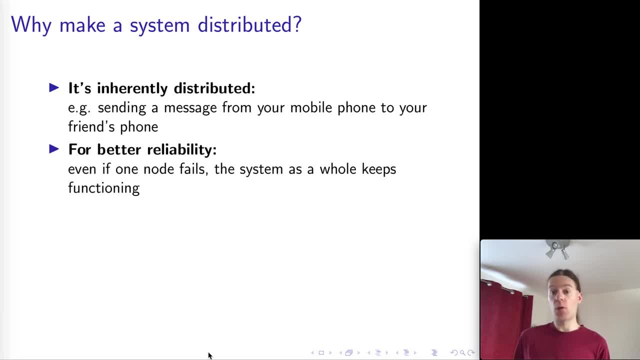 interested in distributed systems, But there are many other reasons as well. So another good reason for being interested in distributed systems is that you can't just send a message from your phone to your friend's phone. The other reason for being interested in distributed systems is that it actually allows us to make 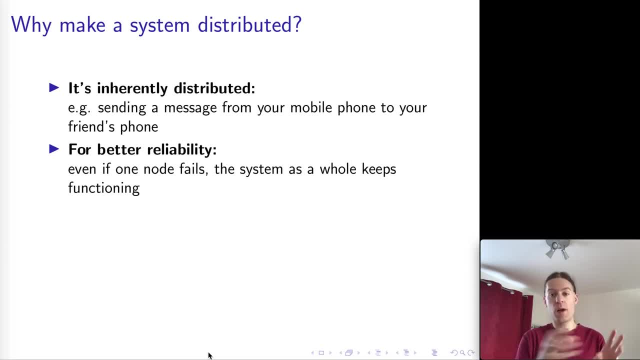 systems more reliable, And the reason for this is say you have multiple computers which are each performing part of some job. If one of those fails, maybe one of them has to be rebooted, for example, or one of them has a hardware failure, then maybe the remaining 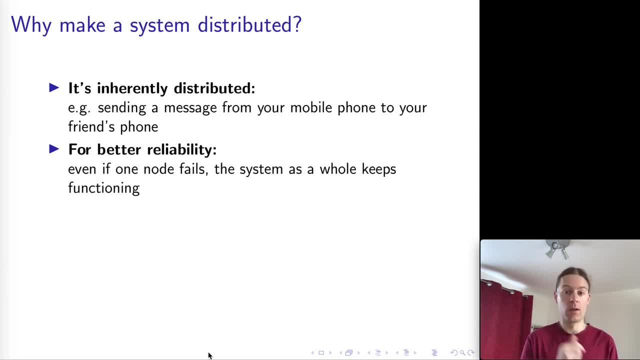 computers can take over the work from the failed computer, And so now this allows the system as a whole to continue functioning, even though one of the computers involved in this has actually gone down. Another reason we might want to make systems distributed is for better. 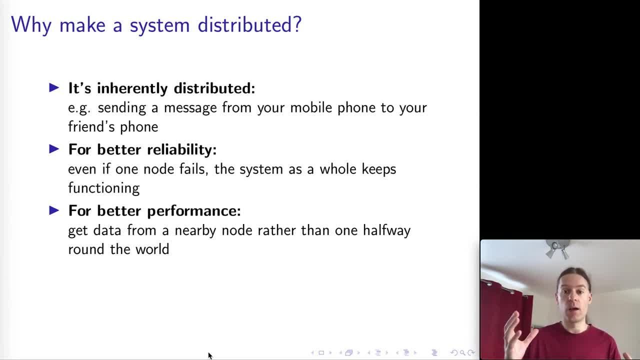 performance. So, for example, in internet distributed systems, you might have users all around the world. You might have some users in the UK, some users in the US, some users in New, Zealand, some users in South Africa, wherever- And there are large distances between these different places. 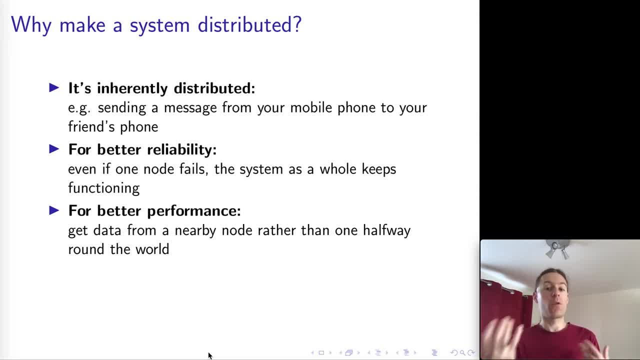 And so network communication from one of these places to the others is always going to take a little- while You're talking, at least 100 milliseconds, simply because of the speed of light that it takes for communication to travel from one continent to another. And so one reason why people are interested in distributed systems is to make systems. 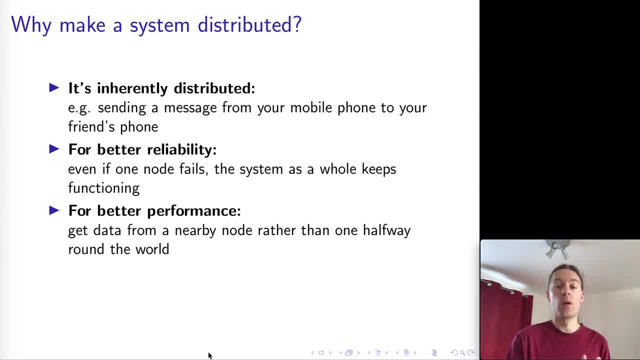 faster by putting data closer to where the people are. So if you have some users in multiple different continents, you can have computers in multiple different continents, And if you have each user communicating with the computer that is most local to them, then you avoid the long distance intercontinental communication. 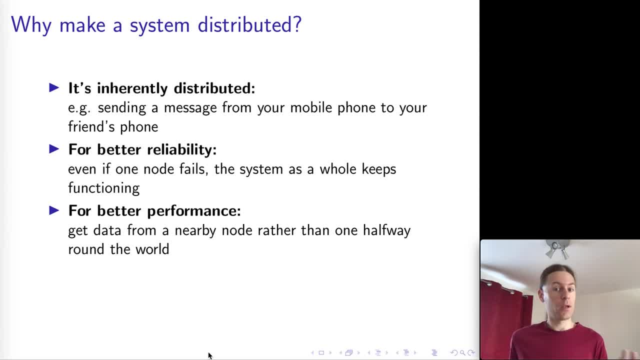 as part of the delays that are added to their communication. So making systems distributed allows us to make them faster, potentially. And finally, another reason why people build distributed systems is to solve bigger problems than they could with a single computer. So some computing problems are simply very large scale. So think of scientific computing. examples. 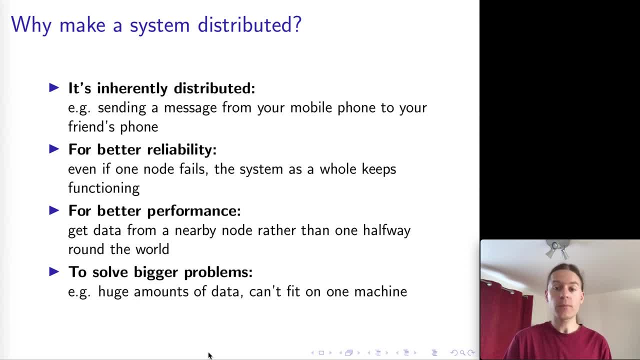 like, for example, the CERN, the particle accelerator in Switzerland. that includes the Large Hadron Collider. They have a vast computing infrastructure involving a million CPU cores and god knows how many hard disks, in order to just take all of the data that they're gathering from. 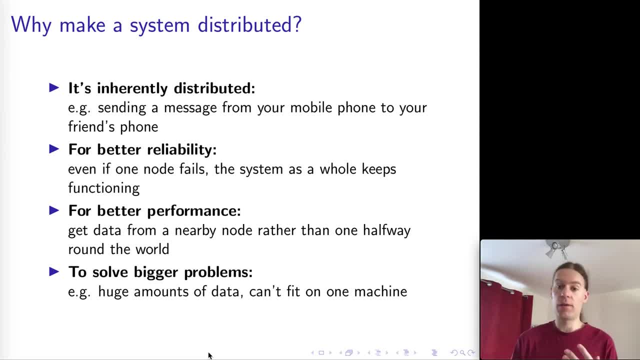 the particle accelerator and process it and analyze it and try to use this to discover new particles, for example. Now you this, this scale of task would simply be not be possible to achieve on a single computer, because there is no supercomputer that is big enough to be able to handle these vast volumes of data. So 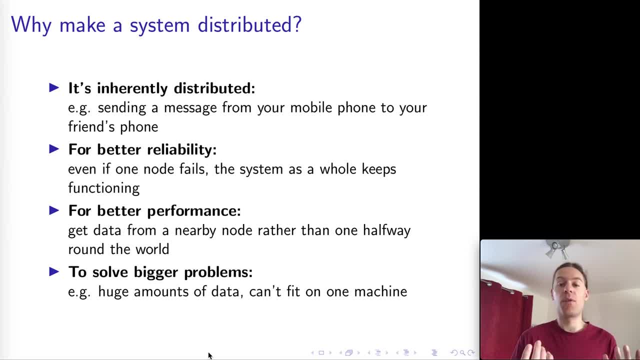 simply solving this problem of analyzing such large volumes of data has to be done on a network of lots of small computers, and those computers have to distribute the work amongst them, and they have to work together in order to achieve the tasks that the scientists are trying to do. 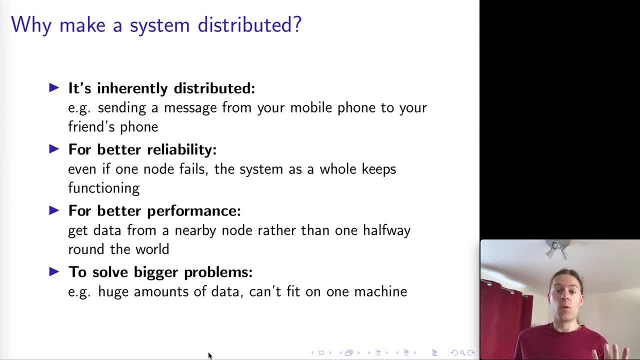 Thank you so much And so Thank you so much. This is really another key area in which we can use distributed systems is to solve bigger problems. This is really another key area in which we can use distributed systems is to solve bigger problems. Now, those are the advantages of making systems distributed. There are, unfortunately, some significant disadvantages as well. 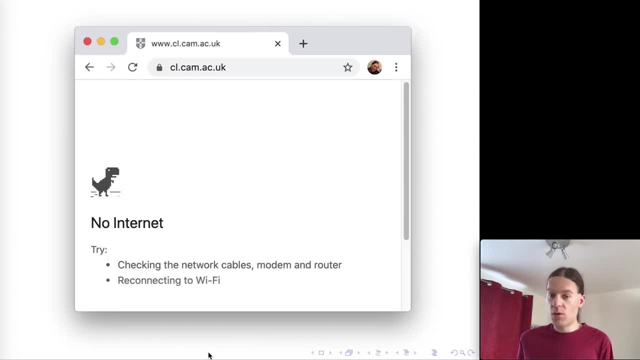 Now, those are the advantages of making systems distributed. There are, unfortunately, some significant disadvantages as well, And the main disadvantage that you will be well familiar with is whenever you're trying to do something over a network, that network might not be working for some reason. 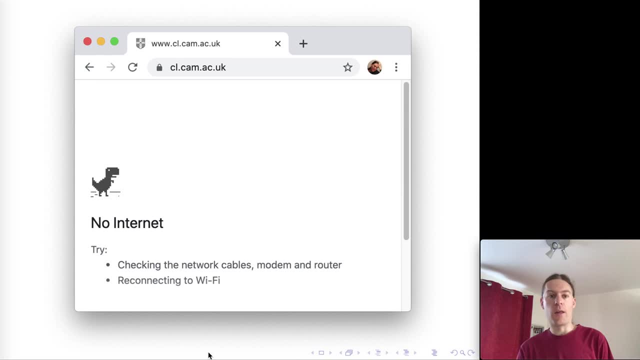 and so. So that will also figure out. do seize more data, and so everyone has experienced what it's like to solve problems with a computer and have to use a lot of other stuff. So everyone has experienced what it's like for the internet to be down or for your Wi-Fi signal to be weak, or for you're in some rural part of the country and your cellular data signal is weak and you're trying to load a map or something like that. 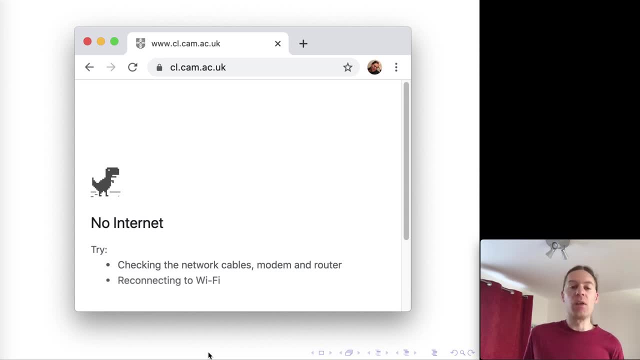 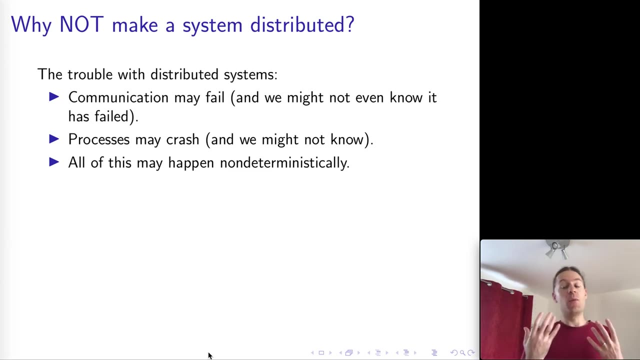 Everyone has experienced this kind of frustration before, and well, the study of distributed systems is all about the study of such frustrations. So we assume, whenever we are building a distributed system that involves communication over a network, that networks are not perfectly reliable, and so it is always possible for communication to fail. 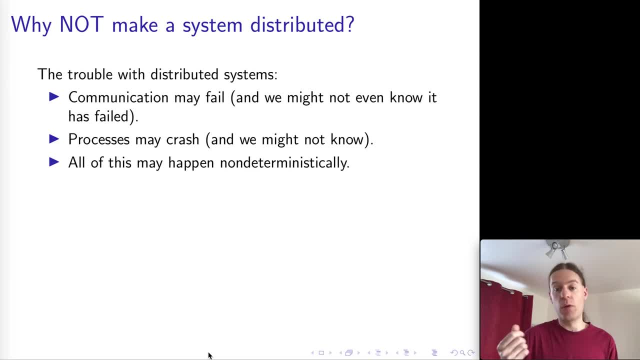 It is always possible that, because if it's a Wi-Fi network, you might be out of range. If it's a wired network, somebody might have unplugged the wrong cable. If it's any type of network, it might just be temporarily overloaded. 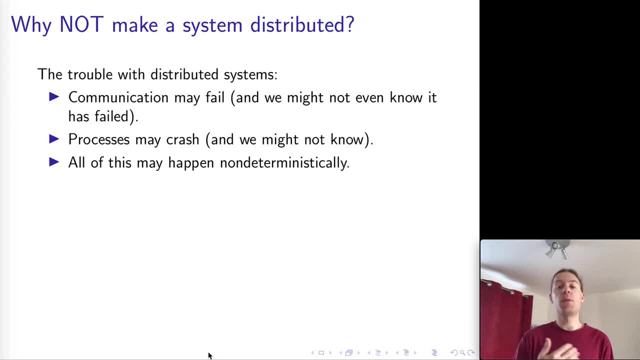 And so it might not work. It might be dropping messages, Maybe even somebody might be maliciously trying to interfere with the network and cause it to drop packets, maybe causing a denial-of-service attack, for example. There are many reasons why communication might not work from time to time. 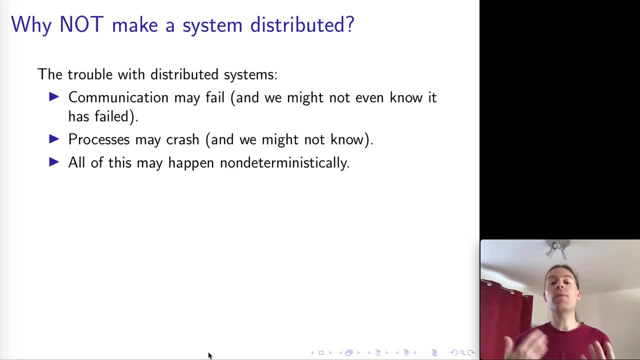 And so we have to build systems that are robust, so that, even if communication is interrupted from time to time, the system as a whole still functions in some correct way, Where, of course, we can define what we mean with correct, but we want it to.